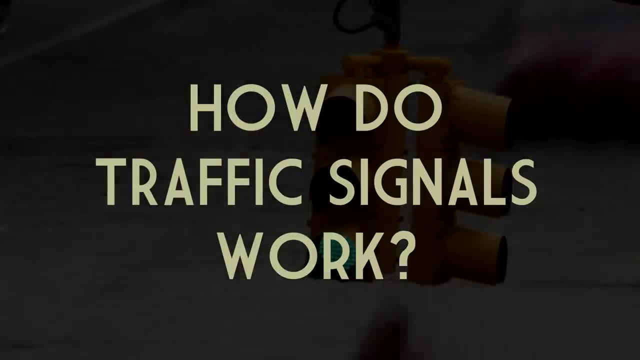 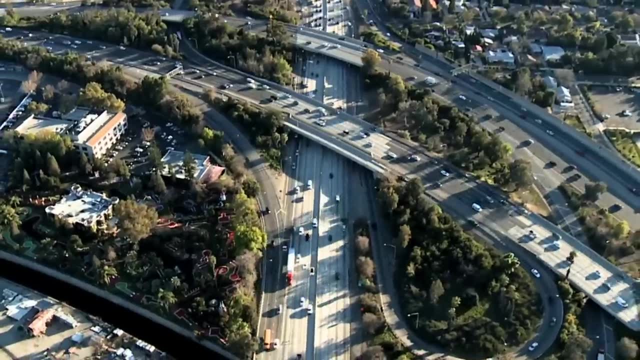 This video is sponsored by Squarespace. More on that later. There are a lot of good analogies between cities and human anatomy, and roadways are no exception. Highways are like the aorta, with a high capacity and single major destination. 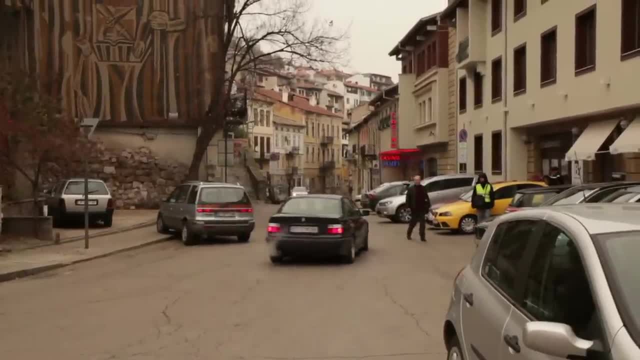 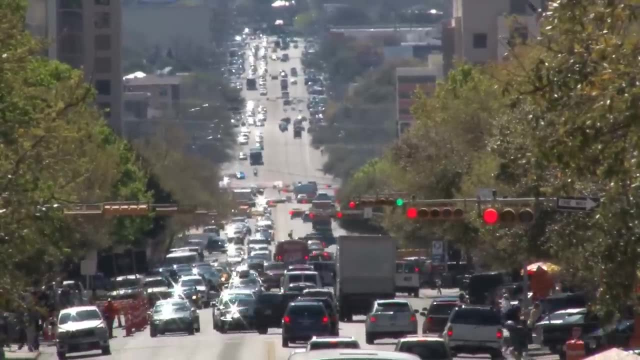 Small collector roads are like the capillaries, with a high capacity and single major destination. not much capacity but a connection to every individual, house and business. And in between are the aptly named arterial roadways, the medium capacity connections between urban centers. 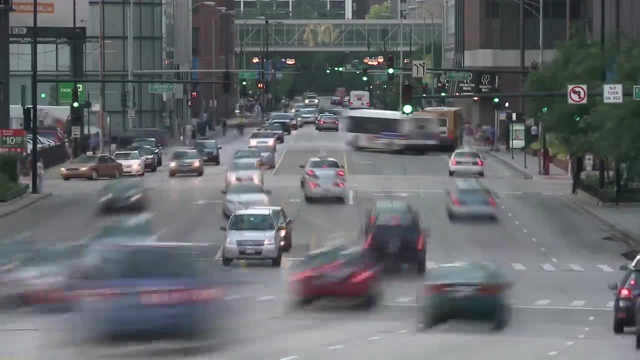 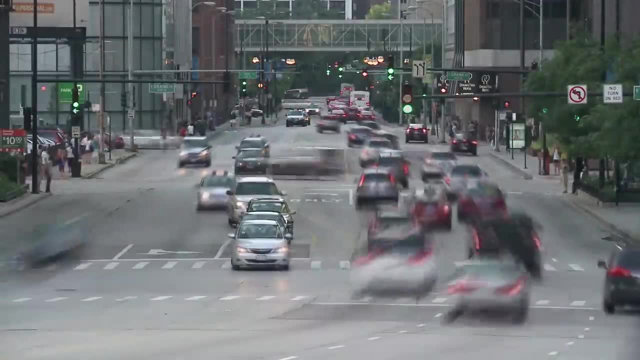 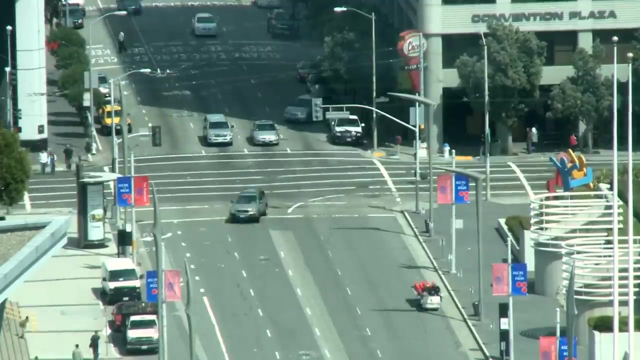 Rather than ramps, overpasses and access roads to control the flow of traffic, arterial roads use at-grade intersections through which only a few traffic streams can pass at a time. We call this interrupted traffic flow for obvious reasons. In most cases, these intersections are the limit to the maximum throughput of the roadway. 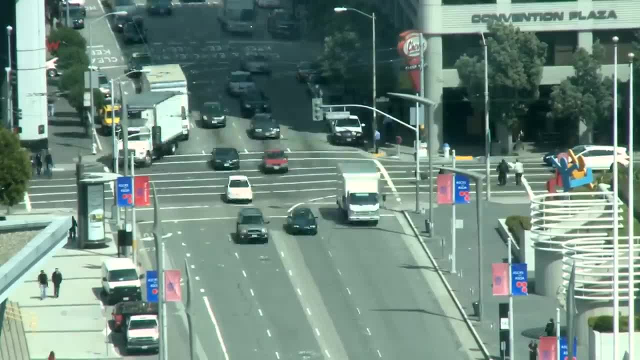 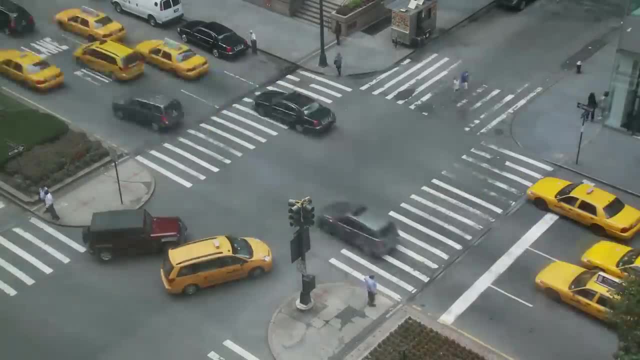 In other words, increasing the number of lanes or speed limit won't have any effect on the overall capacity of the road. The only way to increase the number of vehicles that safely travel from point A to B is to increase the efficiency of the intersection. 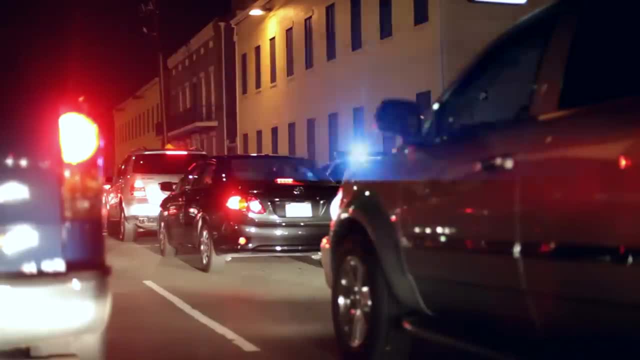 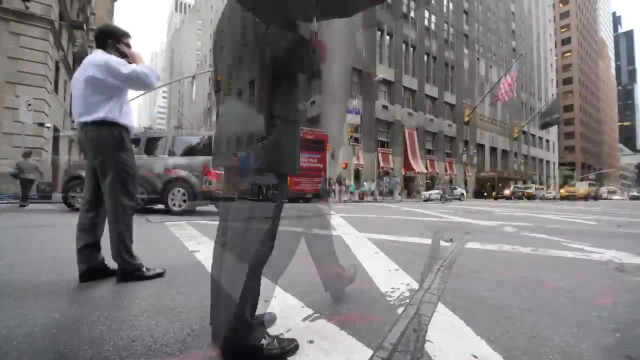 In addition, these intersections are where a vast majority of accidents occur. For these reasons, traffic engineers put a lot of thought and analysis into the design of intersections and how to make them as safe and efficient as possible. Controlling the flow of traffic through an intersection, otherwise known as a traffic 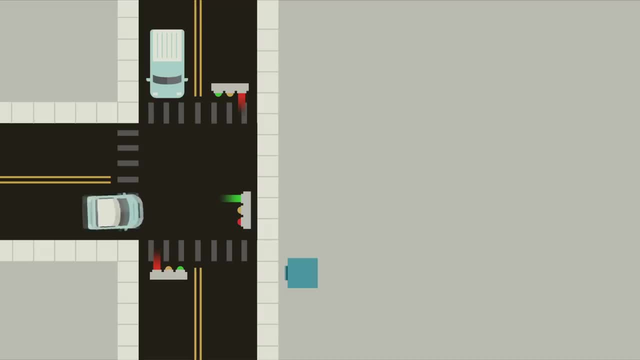 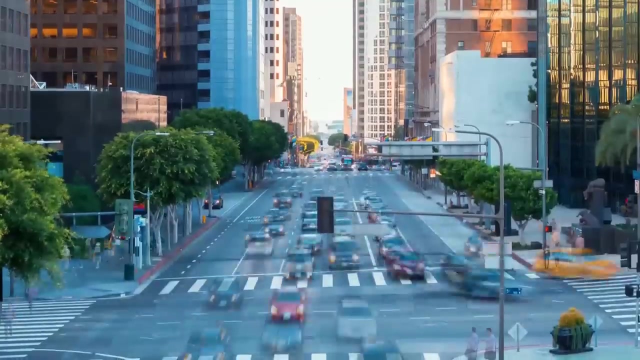 lane is an enormous challenge and almost always requires a compromise of numerous conflicting considerations, including space, cost, approach, speed, cycle time, site distance, types and volumes of traffic, and human factors like habits, expectations and reaction times. Intersections also need to be rigidly standardized so that when you come to an unfamiliar one, 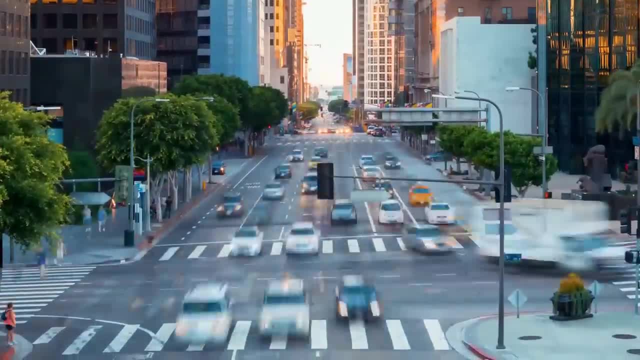 you already know your role in the careful and chaotic dance of vehicles and pedestrians. From a throughput standpoint, the ideal intersection is a traffic lane. In other words, a traffic lane is a traffic lane. This means that any traffic that passes through the intersection would cause no interruption. 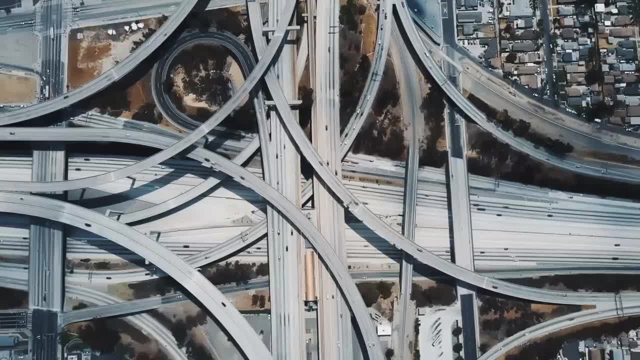 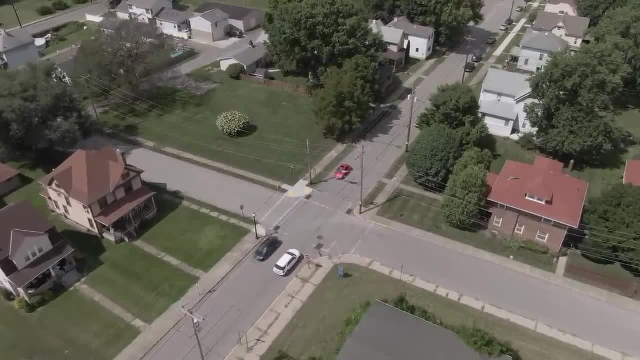 to flow whatsoever, But you can't put a high-five interchange on every city block. On the other hand, simple signs are cost effective and don't require any extra space, but they can't handle a lot of volume because they create an interruption for every single vehicle. 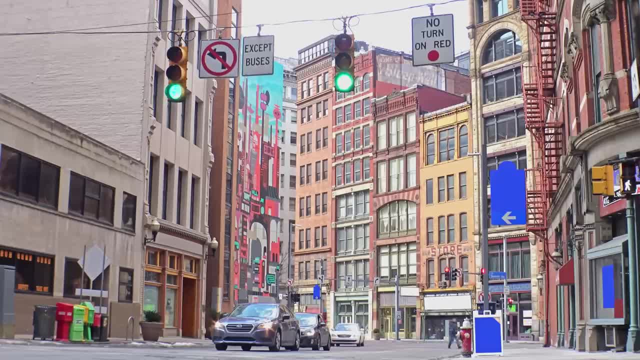 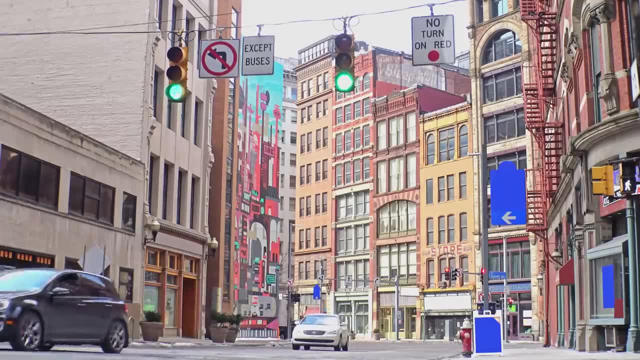 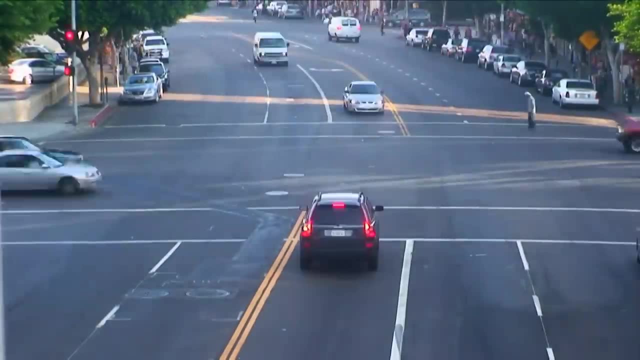 passing through the intersection, You can see why traffic signals are so popular. They aren't a panacea for all traffic problems, but they do offer a very nice balance of the considerations we discussed before: Relatively low costs, Minimal space requirements and the ability to handle large volumes of traffic with only some interruption. 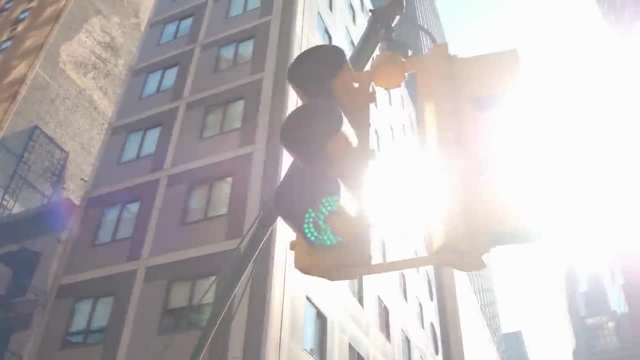 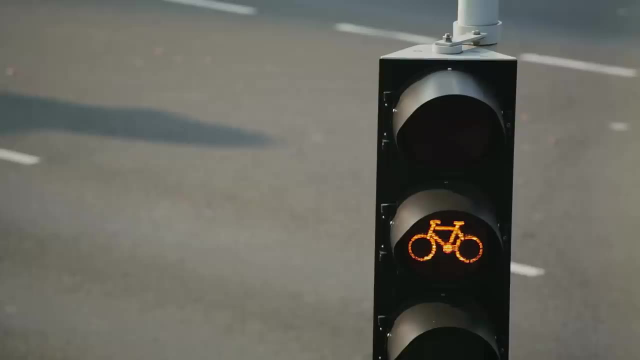 In their simplest form, traffic signals are a set of three lights facing each lane of an intersection. When the light is green, that lane has the right-of-way to cross. When the light is red, they don't. The amber light warns that the signal is about to change from green to red. 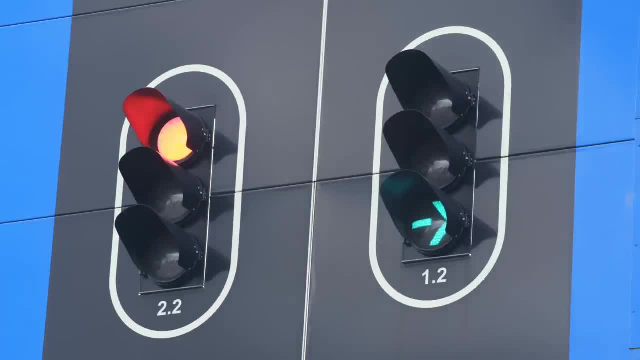 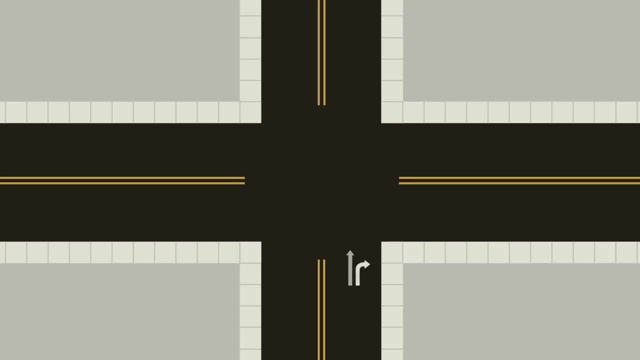 Beyond this basic function, traffic signals can take on innumerable complexities to accommodate all kinds of situations. Let's take a look at a typical intersection here in the US to show how they work. At each approach to an intersection there are three directions vehicles can go, called movements right through or left. 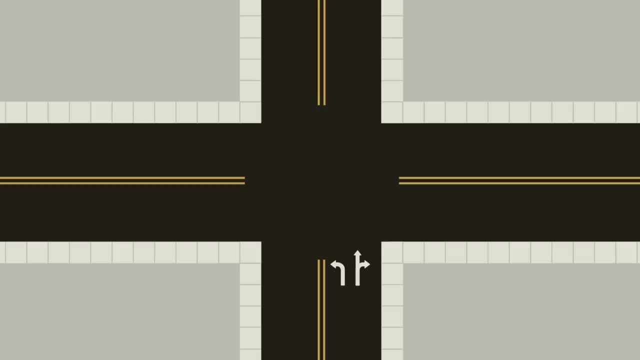 Right and through are usually grouped together as a single movement. so a typical four-way intersection has eight vehicle and four pedestrian movements. These movements can be grouped into phases of the traffic signal. For example, the left-turn movements on opposite approaches can be grouped into a single phase because they can both go at the same time without conflicts. 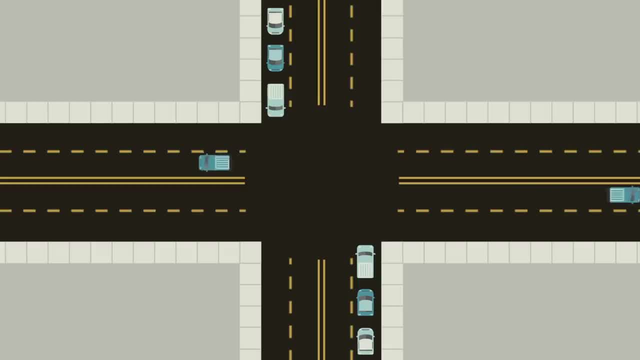 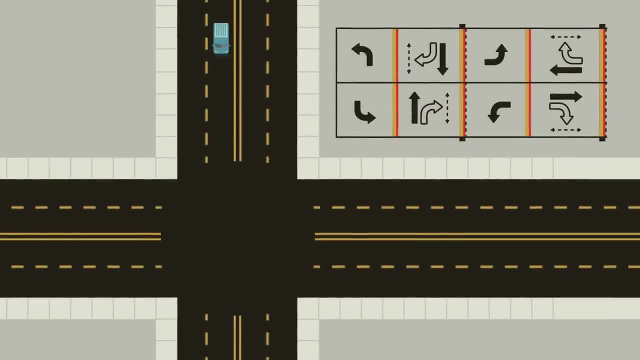 Traffic engineers use a ring and barrier diagram to sketch out how different phases of the signal are allowed to operate. Here's the ring and barrier diagram for our example intersection. The first phase is the major street left turns. then the major street vehicle and pedestrian through movements, a barrier to clear the intersection. the minor street left turns. 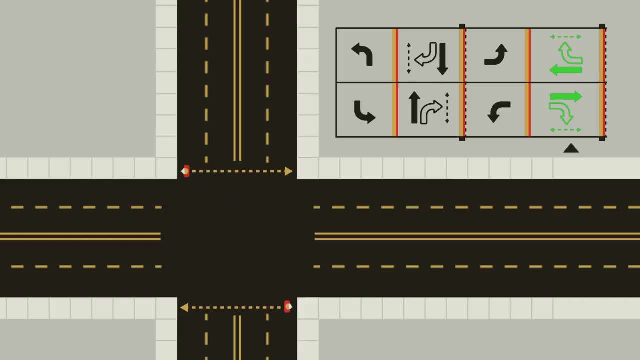 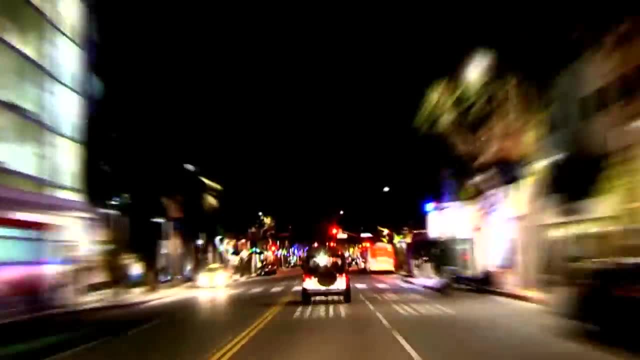 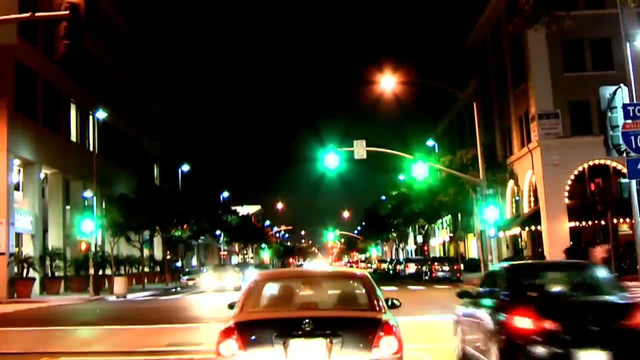 the minor street- vehicle and pedestrian through movements and finally, another barrier before the cycle starts again. There are an endless variety of phasing arrangements that traffic engineers use to accommodate various intersection configurations and traffic volumes for each movement. Even the simple decision of whether to use protected or unprotected left turns. 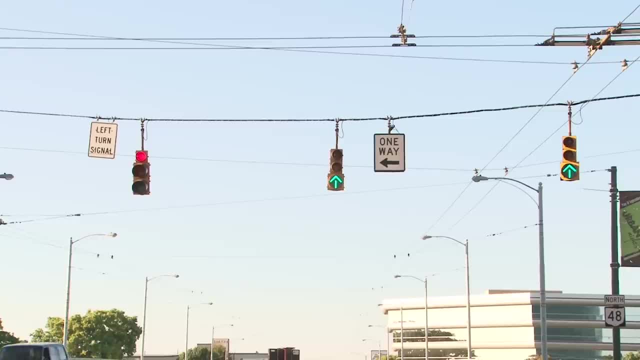 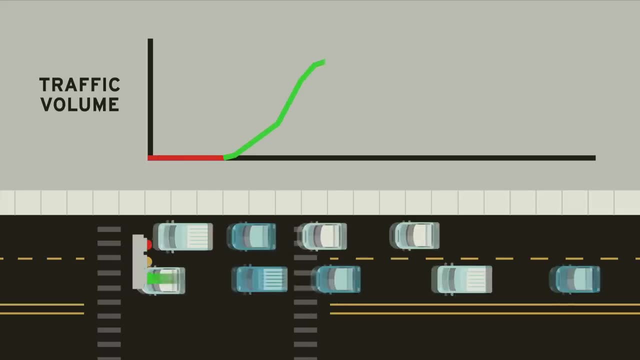 takes a significant amount of analysis and consideration. Another important decision is how long each sequence of a phase should last. Ideally, a green light should last at least long enough to clear the queue that built up during the red light. This isn't always possible. 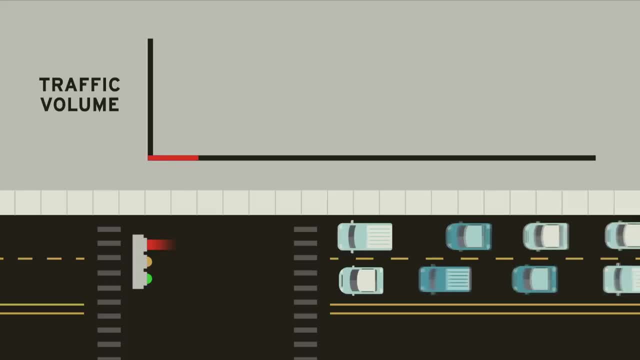 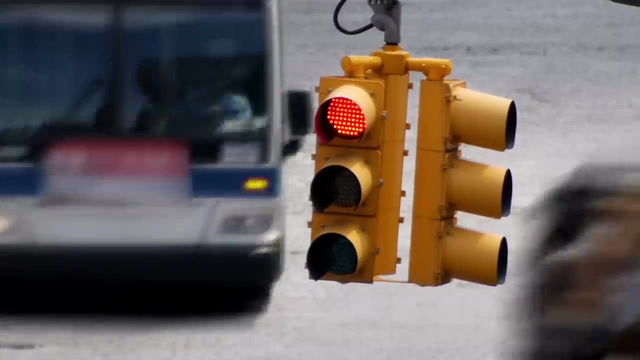 especially during peak times on busy intersections. In these cases, where the intersection is saturated, the green light might be extended for each phase to minimize the startup and clearance times, which are periods when the intersection isn't being utilized to its maximum capacity. The amber light needs to last long enough for a driver to perceive the warning and. 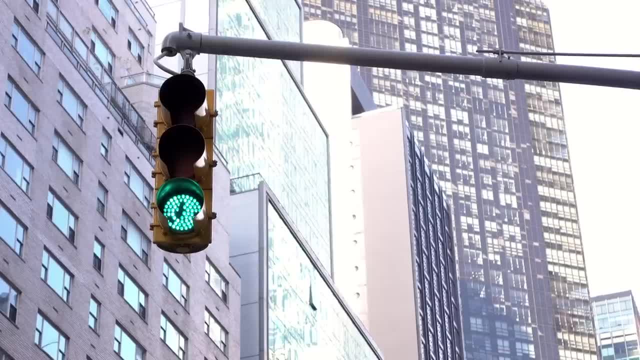 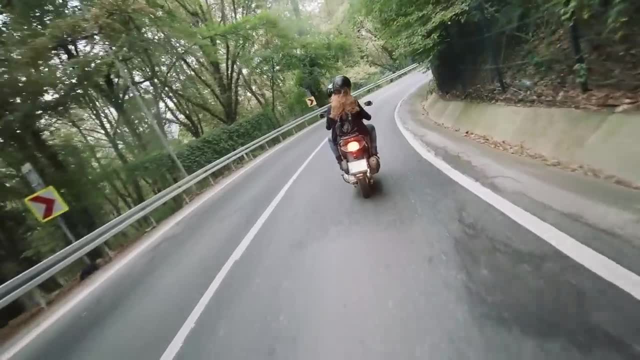 decelerate their vehicle to a stop at a comfortable rate. One second for every 10 miles per hour, or so. 16 kilometers per hour on the speed limit is a general rule of thumb, but traffic engineers also take into account the slope of the approach and other local considerations when setting. 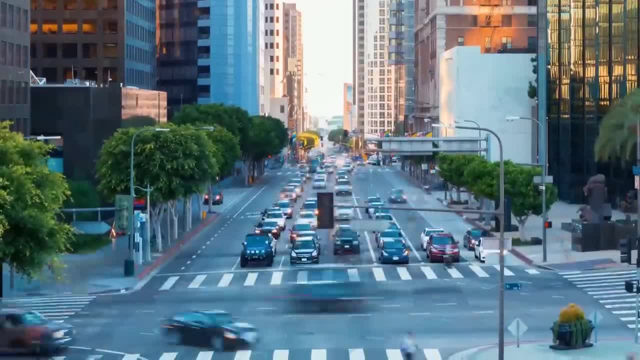 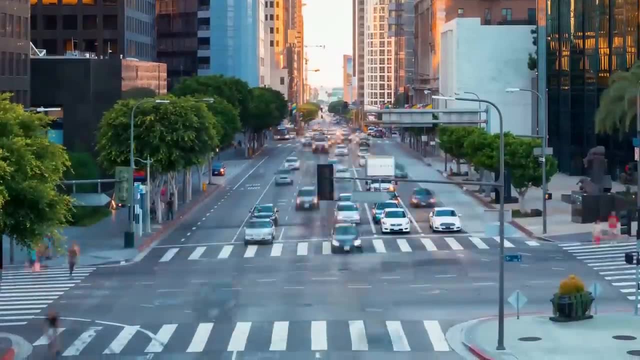 the timing for yellow lights. In most places in North America you're allowed to enter an intersection for the full duration of a yellow light, which means there needs to be a time when all phases have a red light to allow the intersection to clear This clearance interval. 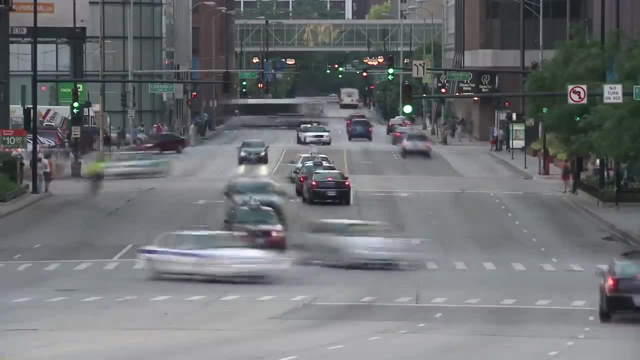 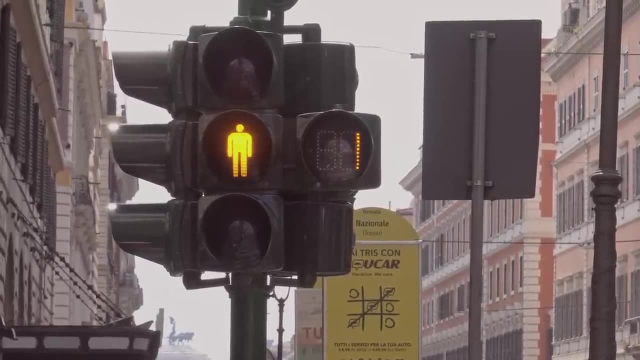 is usually about a second, but can be adjusted up or down based on speed limit and intersection size. So far we've only been talking about signals on a set timing sequence, but most traffic signals these days are more sophisticated than that. Actuated signal control is the term we use for 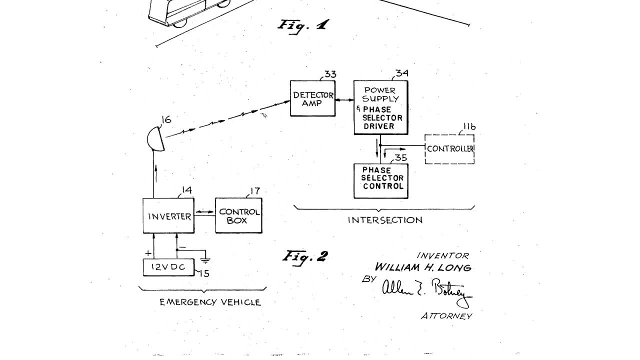 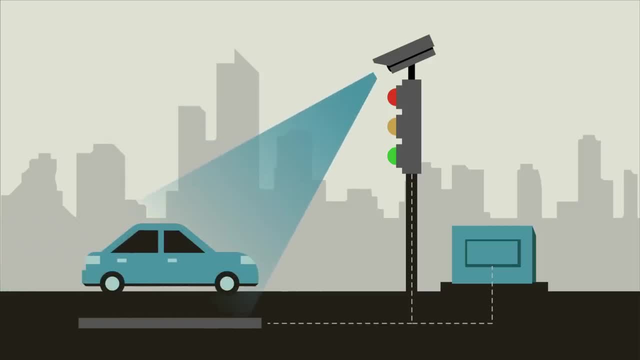 signals that can receive input from the outside and use that information to make decisions about light, timing and sequence on the fly. These type of signals rely on data from traffic detection systems. These sensors can be embedded cameras or radars, but most commonly they're inductive. 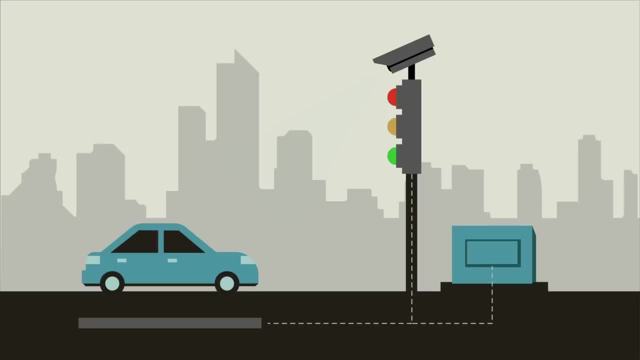 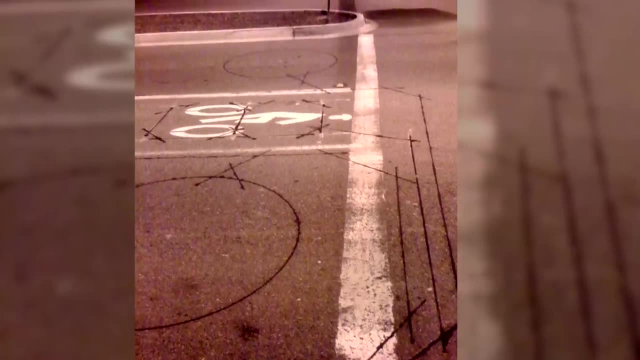 loop sensors embedded into the road surface. They are essentially the same type of sensors that are used to measure whether or not a car or truck is present, sometimes to the annoyance of bicycles, scooters and motorcycles that may be too small to trigger the loop. Whatever the type of sensor, 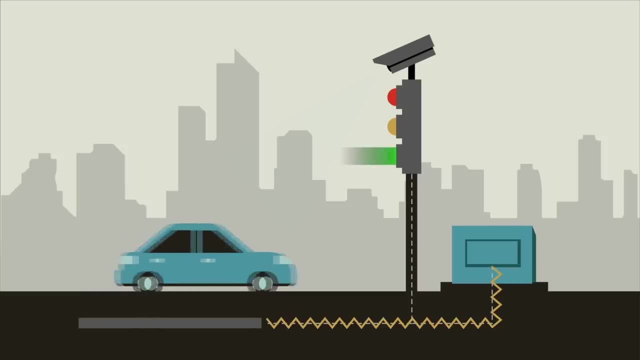 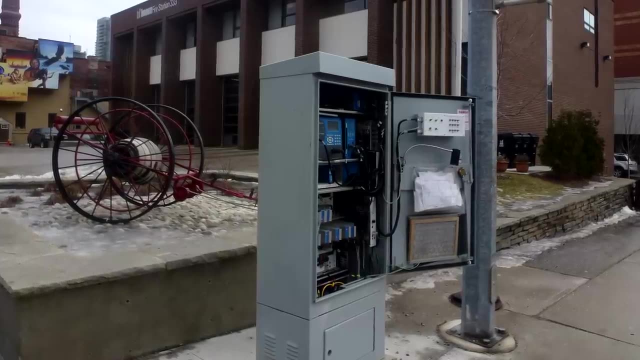 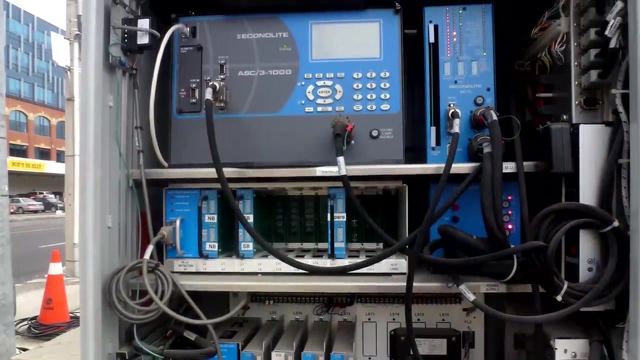 they all feed data into an equipment cabinet located nearby. You've probably seen hundreds of these cabinets without realizing their purpose. Inside this cabinet is a traffic signal controller, essentially a simple computer that is programmed with specific logic to determine when and how long each light will last, based on the information from the sensor. This computer is essentially 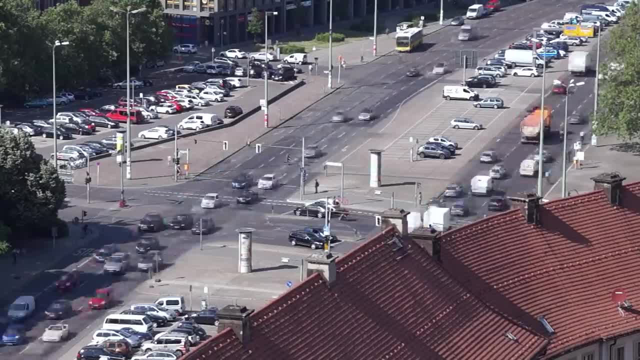 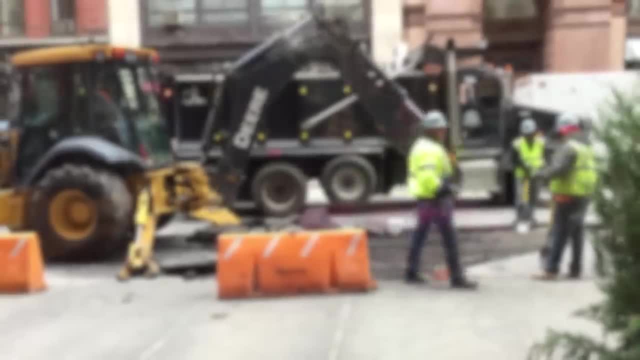 the same as a traffic signal controller. Actuated control gives a traffic signal much more flexibility to handle variations in traffic load, For example, if a nearby road is closed and traffic rerouted through a signal that doesn't normally see such high demand. 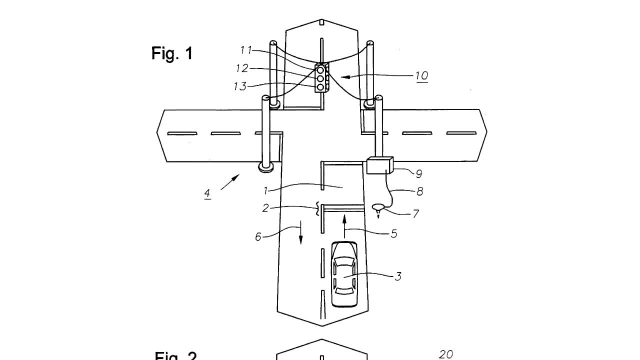 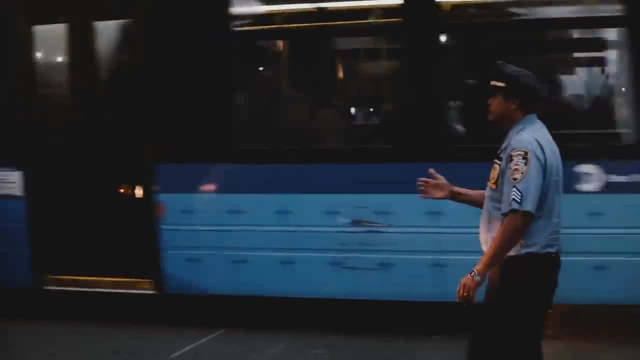 it may need to be reprogrammed before the closure. A light equipped with actuated control will simply see the additional traffic and adjust its phasing accordingly. Same thing with special events like concerts and sports games that create huge traffic demands on irregular schedules and even seasonal. 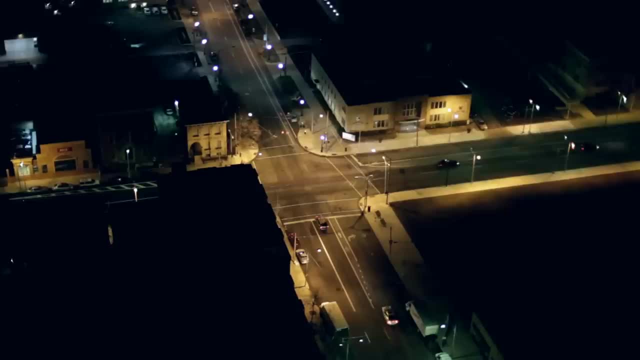 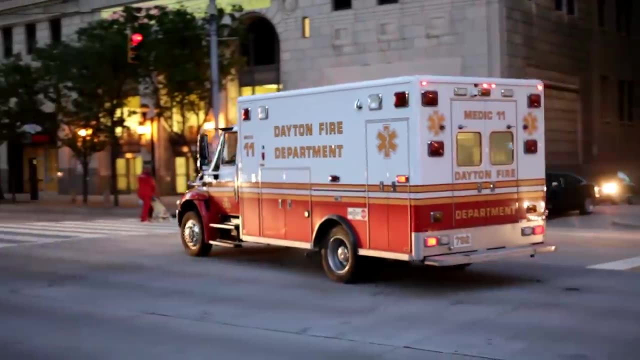 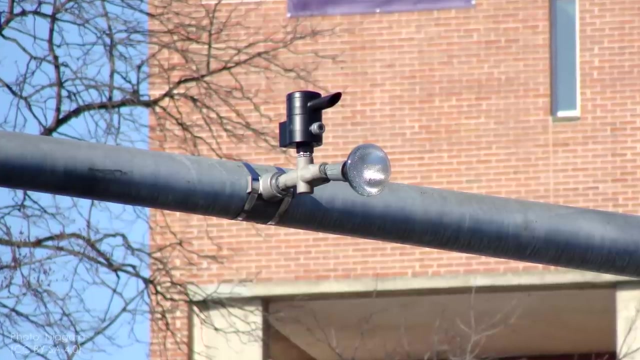 changes in traffic, like in major tourist destinations. Actuated systems can also keep you from waiting at a long light when no one's crossing in the other direction. Finally, actuated control can help by giving priority to emergency vehicles and public transportation, by using specialized detectors like infrared or acoustic sensors that communicate. 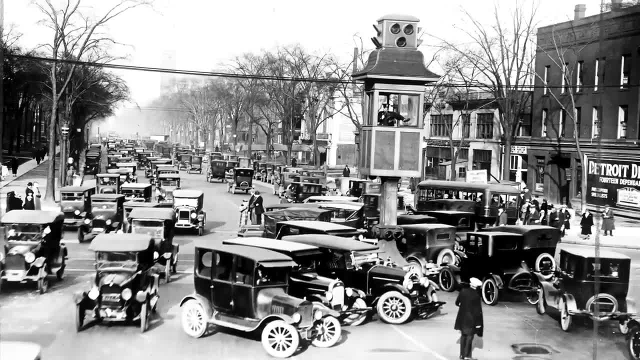 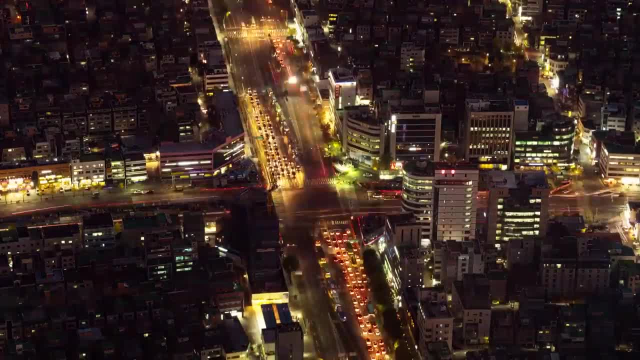 directly with certain types of vehicles. But actuated control isn't the end of the complexity. After all, it still treats each intersection as an isolated entity when in reality each signal is a component of a larger traffic network And each component of the traffic network can have. 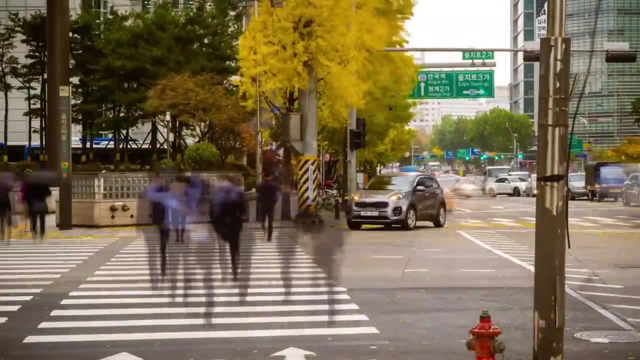 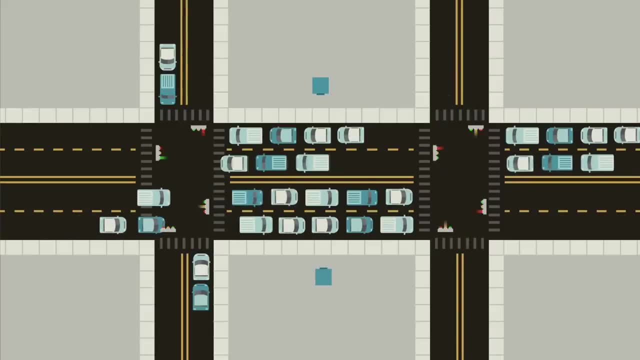 an impact, sometimes a major impact, on other components in the system. Take the classic example of two signals closely spaced in a row on a major roadway. If one signal gives a green but the next one doesn't, cars can back up. If they back up far. 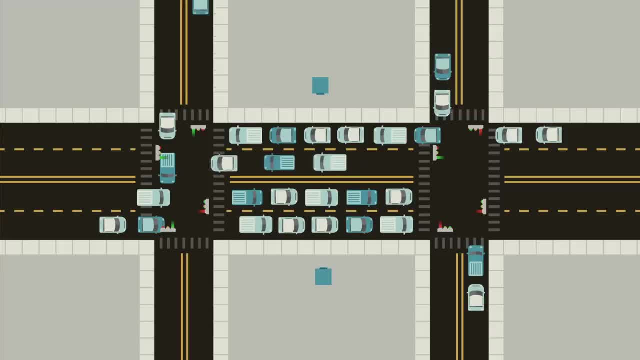 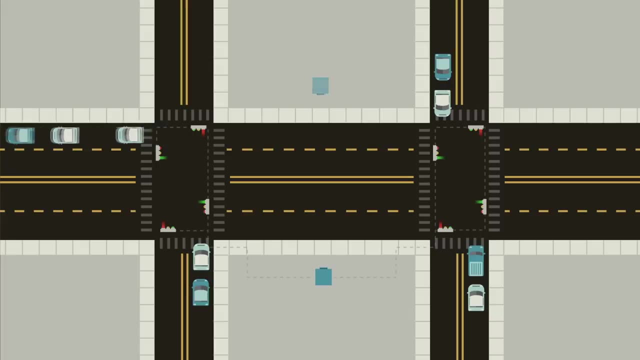 enough, they can sit through multiple cycles at an intersection without being able to pass through until the light beyond clears. It's a frustrating experience for anyone. A signal is interlocked inadvertently, but significantly reducing the capacity of an adjacent signal. One solution to this problem is signal coordination, where lights can not only. 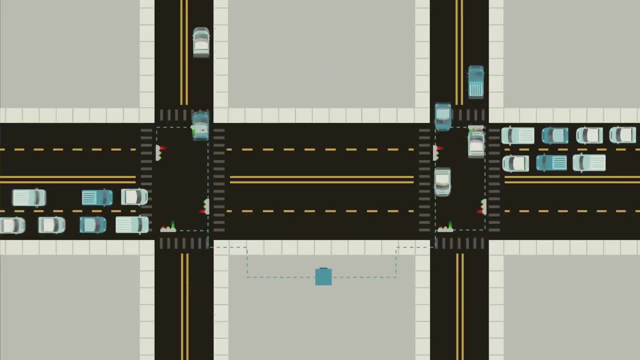 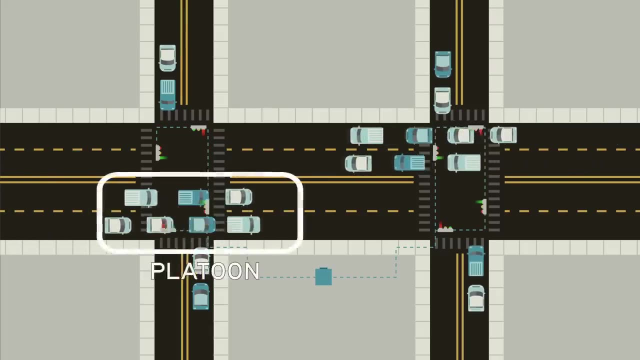 consider the traffic waiting at their intersection, but also the status of nearby signals. This is a very common configuration on long corridors with relatively minor but frequent cross streets. The signals on the major road are timed so that a large group of vehicles, called a platoon by traffic engineers, can make it all the way through the corridor without 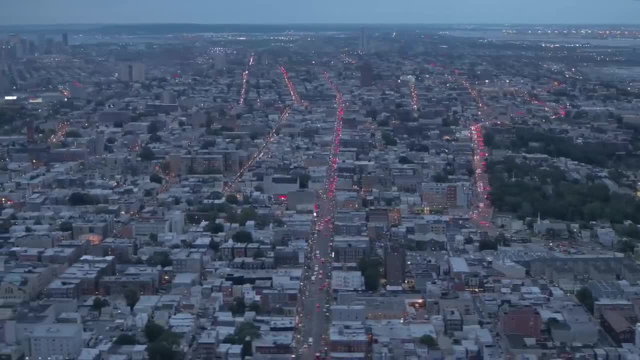 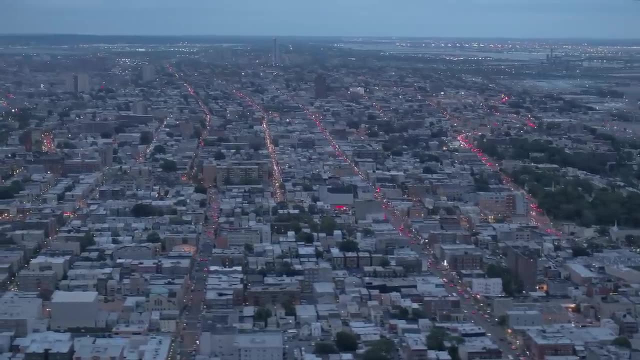 interruption. This type of signal coordination can significantly increase the volume of traffic that can pass through intersections, but it really only works on stretches of road that don't have other sources of traffic interruptions, like driveways and businesses. If the platoon can't. 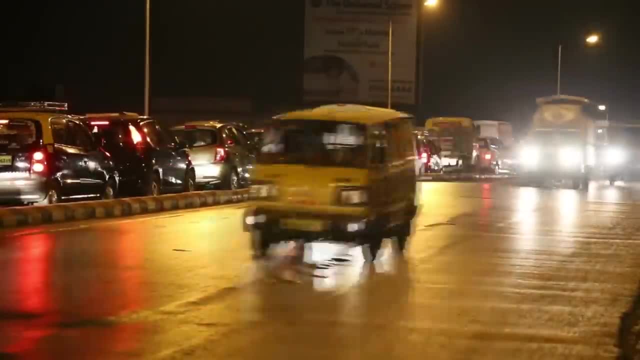 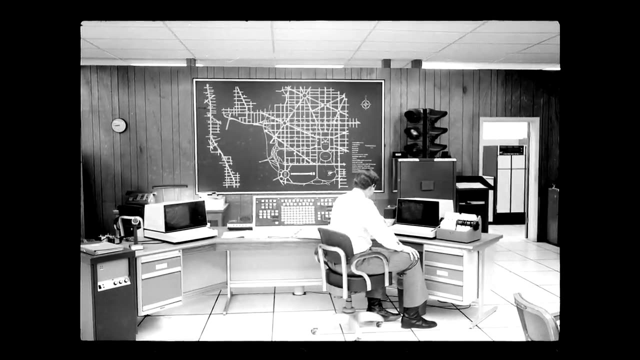 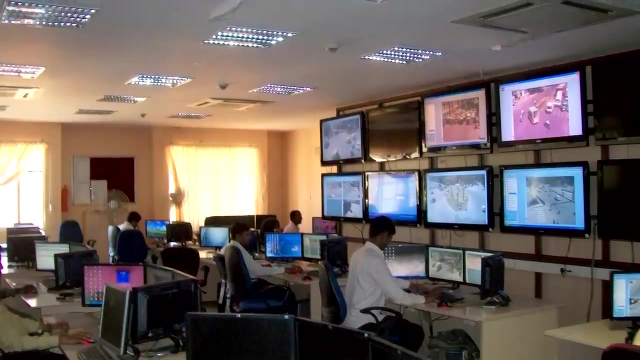 stick together, the benefits of coordinating signals mostly get lost. The obvious next step in efficiency is coordination of most or all the signals within a traffic network. This is the job of adaptive signal control technologies, or ASCT, and adaptive systems Rather than individual groups of lights. all the information from 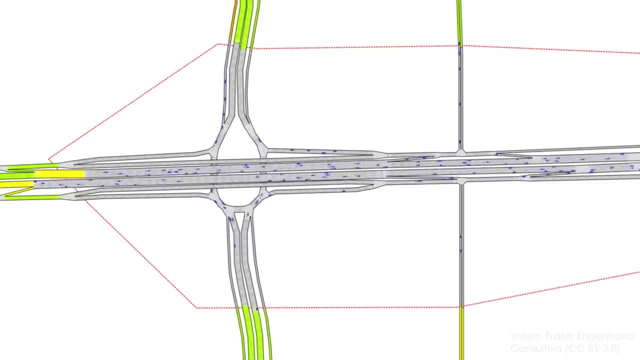 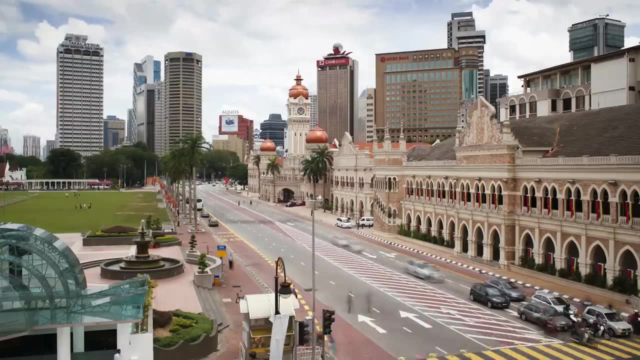 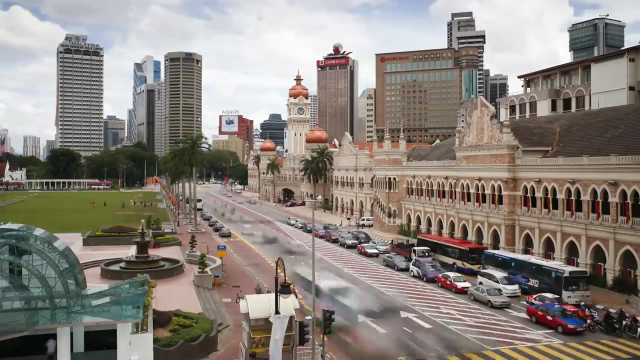 detectors is fed into a centralized system that can use advanced algorithms like machine learning to optimize traffic flow throughout the city. These types of systems can dramatically reduce congestion, but they're only just starting to be implemented in major urban areas. As sensors become more ubiquitous and computing power increases, traffic management may slowly 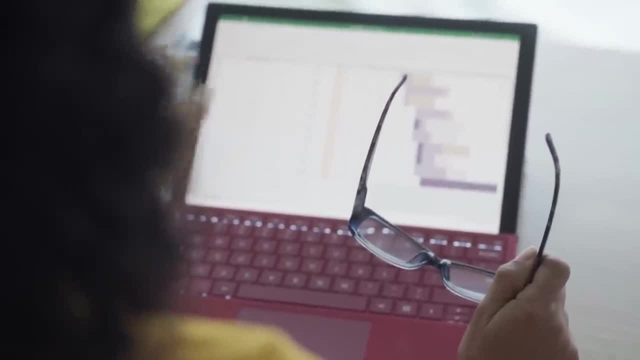 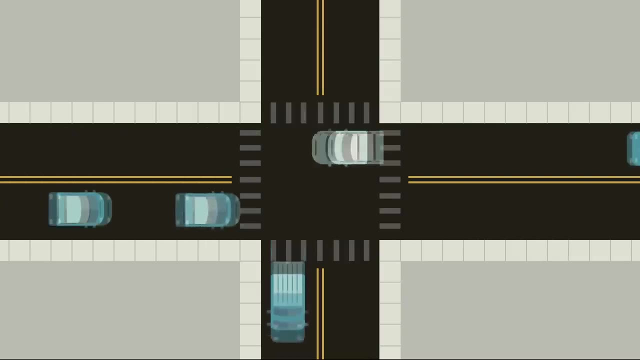 but surely be relegated from civil engineers to software developers and data scientists. On the complete opposite side of centralization, many believe that self-driving cars are the next revolution in traffic management. If every vehicle could communicate and coordinate with every other vehicle on the road. 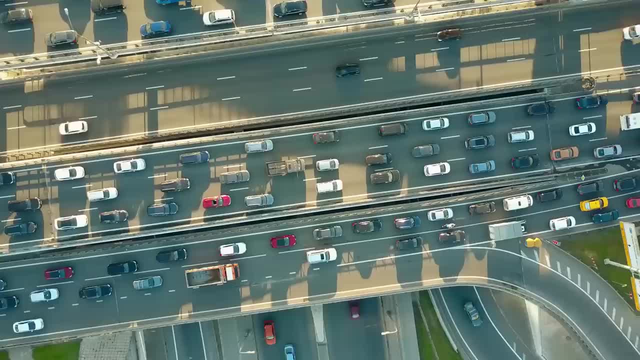 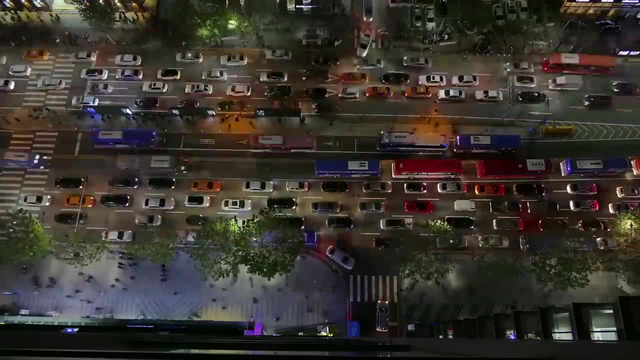 interrupted traffic control could eventually become a thing of the past, But don't get your hopes too high. In dense urban areas, traffic congestion is often self-limiting, Especially during peak times. for every one person on the road, there are many more at. 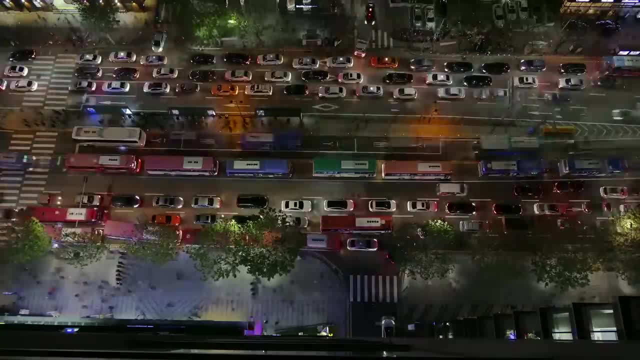 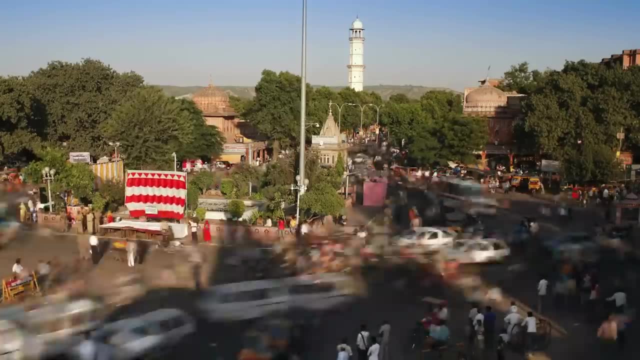 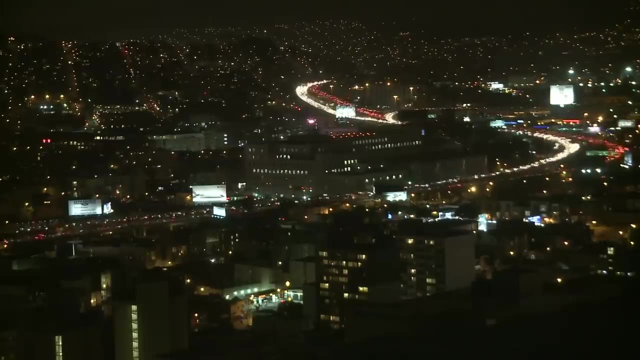 work or at home, waiting for the congestion to clear up before they head out. This latent traffic demand means that any increase in capacity will quickly be filled up with more traffic, bringing the congestion back to the same level it was before. However, we accommodate it. now or in the future, traffic will continue to be one of the biggest 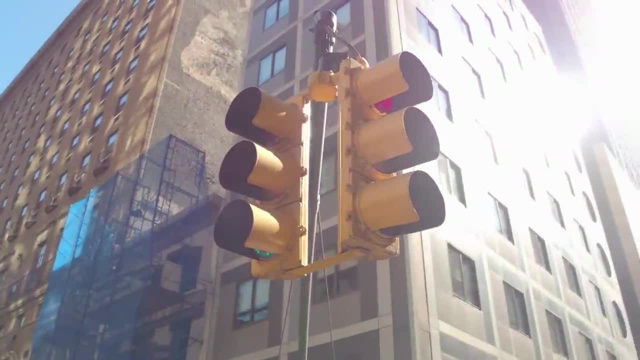 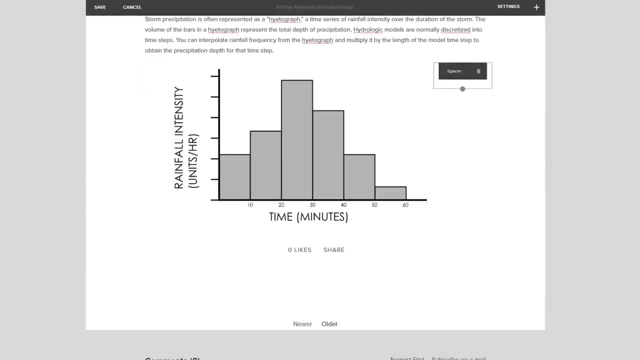 challenges in our urban areas, and traffic signals will continue to be one of its solutions. Thanks to Squarespace for sponsoring Practical Engineering. In a previous video, I asked you for suggestions on my website and got some great feedback. One that I really liked is 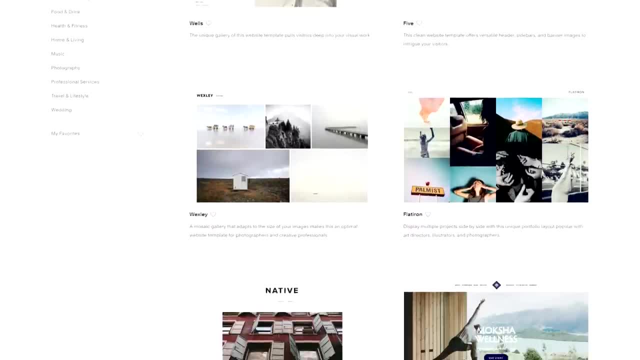 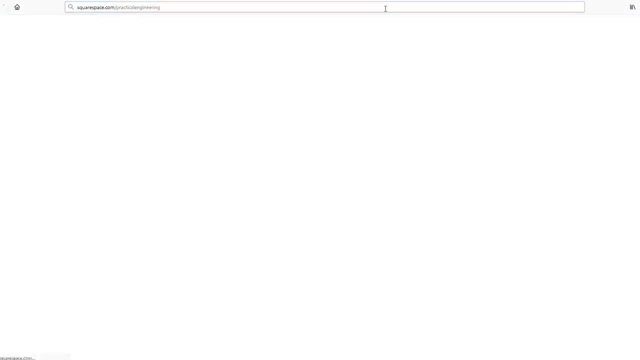 should be more interactive. Squarespace is an all-in-one platform to build a website that doesn't require plugins, updates or patches, And they're offering you a free trial at the link in the description below. Use code Practical Engineering to get 10% off, Just because. 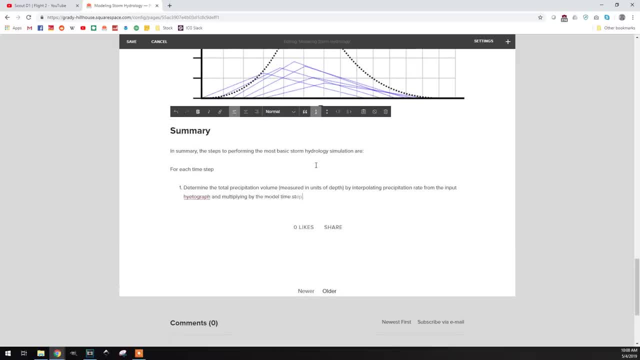 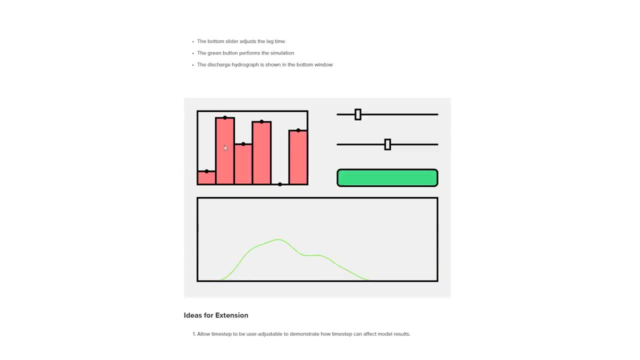 Squarespace is simple to use doesn't mean limitations and features. In fact, I wrote this article explaining how engineers use hydrologic models, and I actually coded a simplified model as a demonstration. Using a code block, I can drop this javascript window directly. 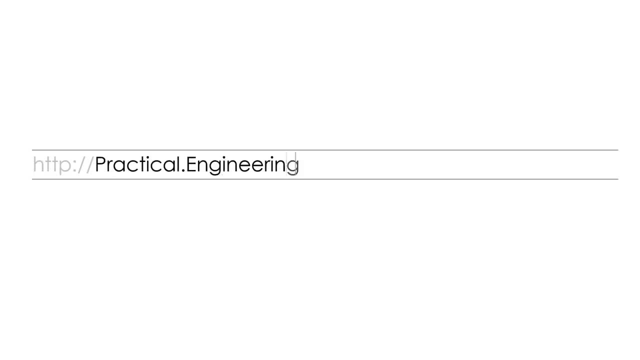 into my article. Go take a look and see for yourself at practicalengineering, And let me know in the comments what other type of stuff you'd like to see me post there, If you've got an idea to share with the world. Squarespace is offering fans of the channel a free. 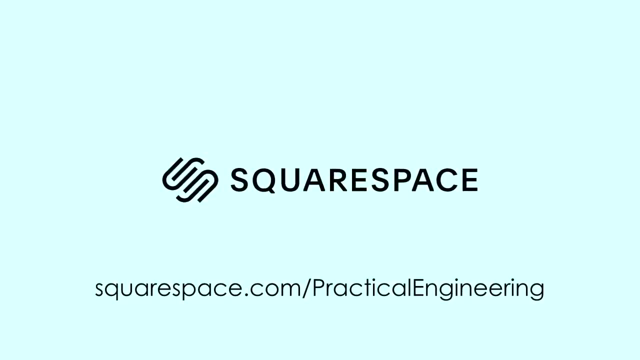 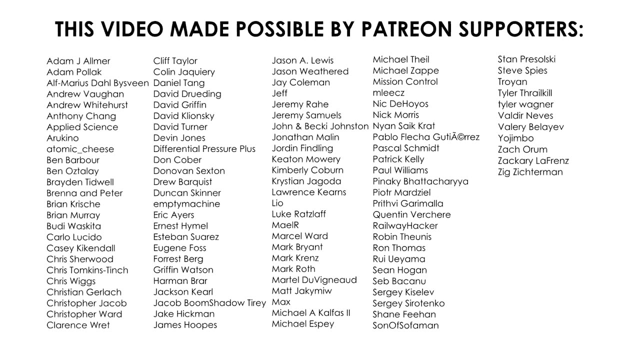 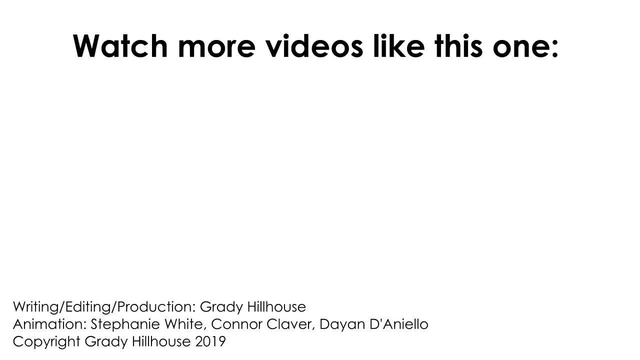 trial at squarespacecom: slash practical engineering or just click the link in the description below. Use code Practical Engineering to get an additional 10% off your first purchase. Thank you for watching and let me know what you think. I'll see you in the next video. 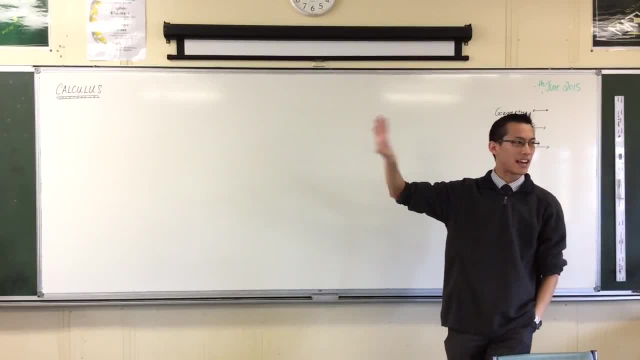 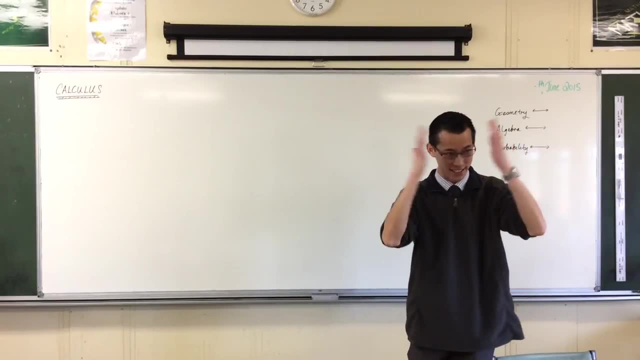 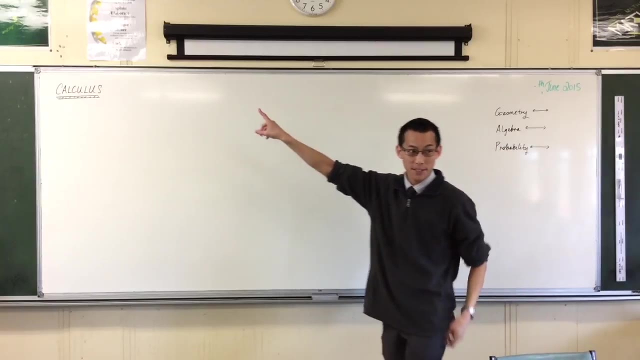 The thing I need to say before we actually begin digging into this is: I know many of you have met this topic already. okay, I just want you to forget everything you have ever heard about this. Just blank slate. okay, The biggest danger, especially with a class like this, is to approach this, this topic, as just like a set of 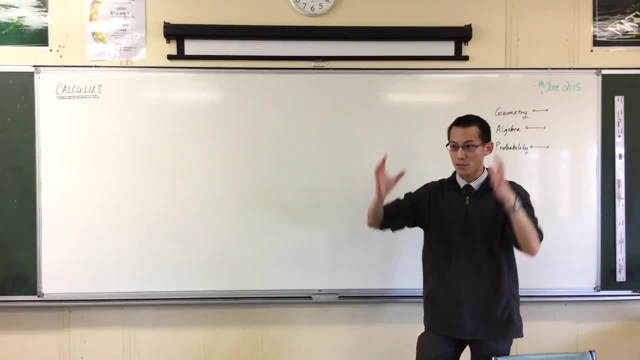 rules, basically Set of rules. memorize the rules, learn how to apply them to. you know hundreds, thousands, maybe situations, and then that's it. You know calculus. Nothing could be further from the truth, okay. 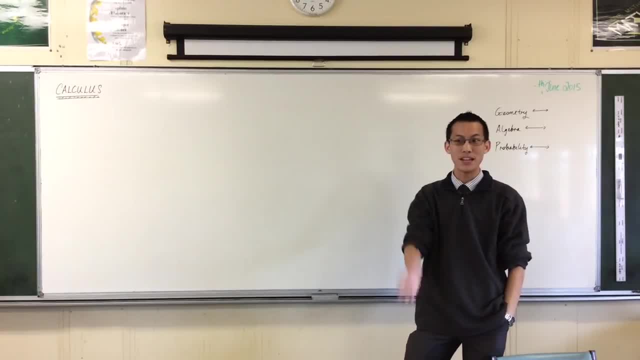 The design and the use of calculus is such a creative process that to just reduce it down to okay, like you will learn rules. you will learn rules. but if learning rules is what calculus is to you, then you don't know what calculus is okay. 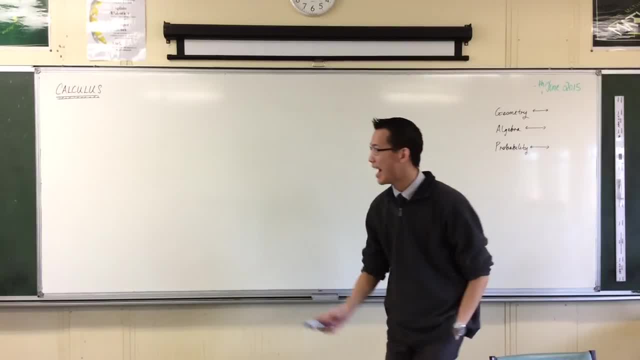 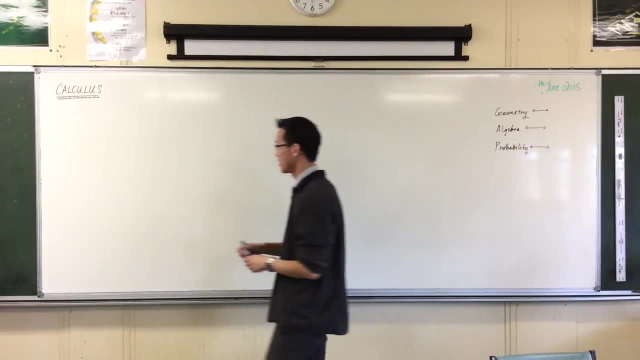 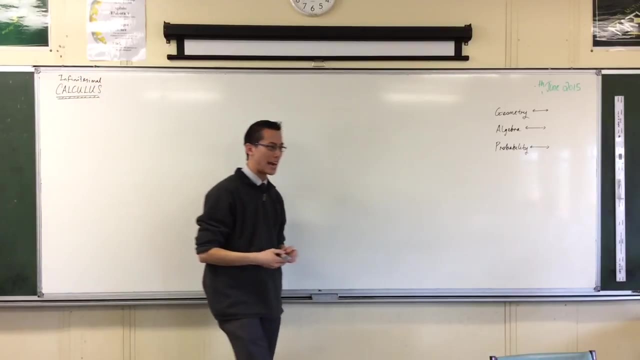 So now pick up your pen and let's think about what this is. Calculus is actually an abbreviation. The full name of calculus is Infinitesimal calculus. Now, the reason why like this is what we're actually going to be doing: infinitesimal calculus.